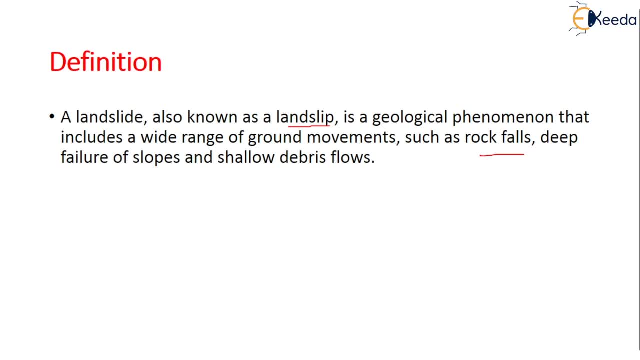 deep failure of slopes and also a shallow debris flows will occur in landslides. Here, the landslides can occur in off-shore coastal and on-shore environments Also, although the action of gravity is a primary driving factor for the landslides to occur. This 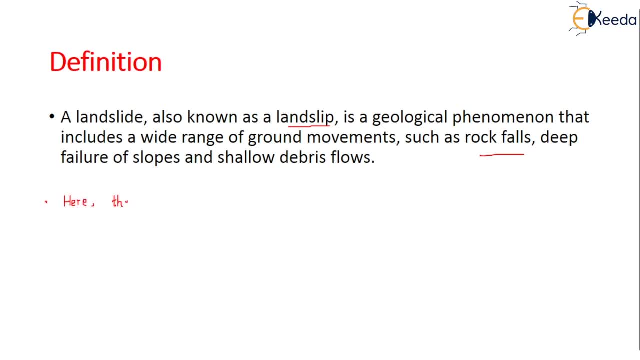 is the insult material. in the final analysis, You will find that returns from normalkilograms or the important point you have to understand. Let me write down- This is the first important point- that landslides can also occur in offshore, coastal and onshore. 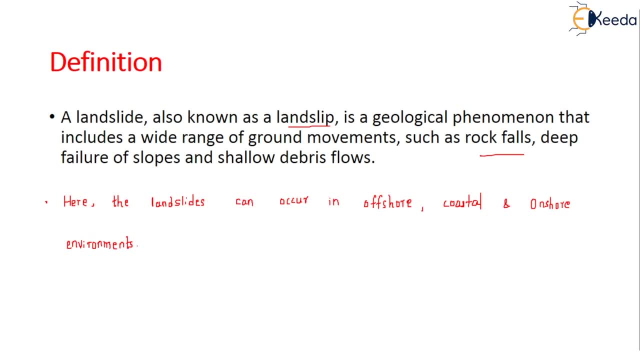 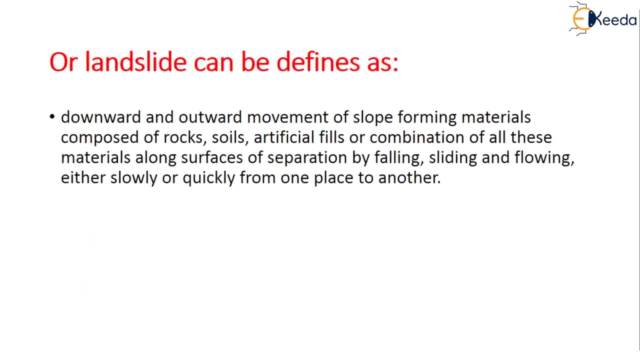 environments. What is the second point? you have to remember What is the primary driving force here? Action of gravity. So the action of gravity is the primary driving force to occur. the landslide. We can also tell that it is downward and outward movement of the slope which is forming the 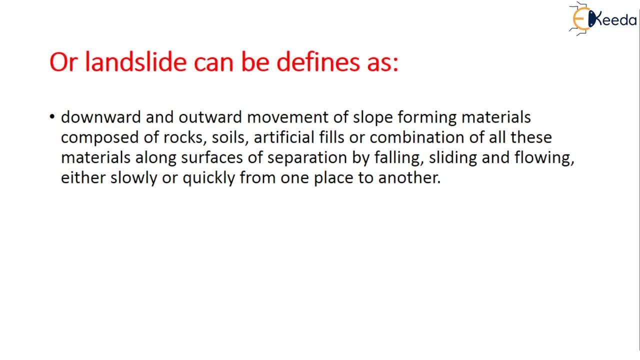 materials composed of rocks, soils, artificial fields or sometimes the combinations of both, one or more. Here there will be separating of falling, sliding and flowing. These are the three important points you have to remember. It may be quite slowly process or sometimes quick. 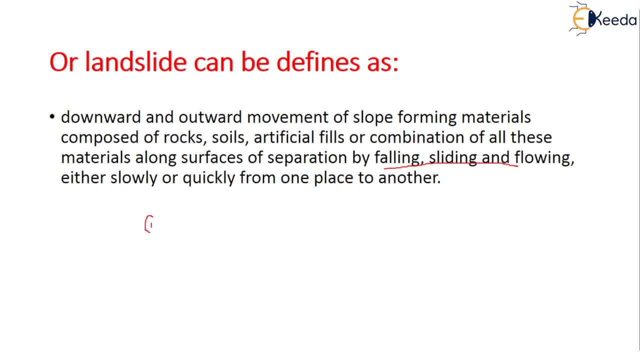 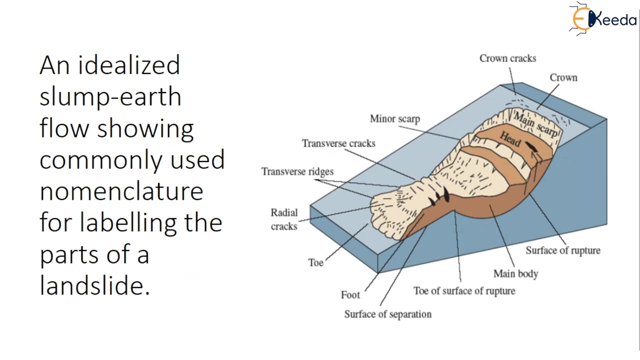 process. What are the three things it may happen? It can be falling process, it can be sliding process or it can be flowing process. So this is the idealized slump earth flow, showing some commonly used nomenclature for labeling the parts of landslide. See, this is the upper part. Uppermost part is called the crown. 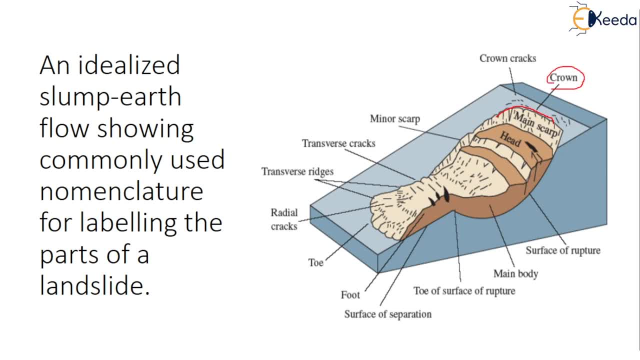 This is very important. We generally know the meaning of crown: the upper part. Similarly, here the upper part is called the crown. So this is the upper part, So this is the upper part, This is the crown, the uppermost part. Here in the crown region, we will see the crown cracks. 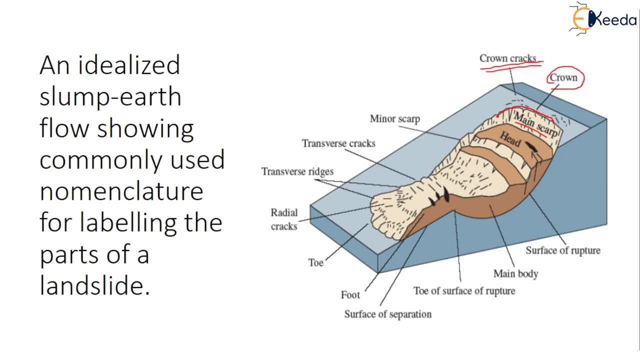 And this region which is associated with the crown is known as main scar And here it is called a head part. the lower of the crown And also the lower surface is called the surface of rupture, where the rupture of the landslide will occur, And this is the main body where the whole rock 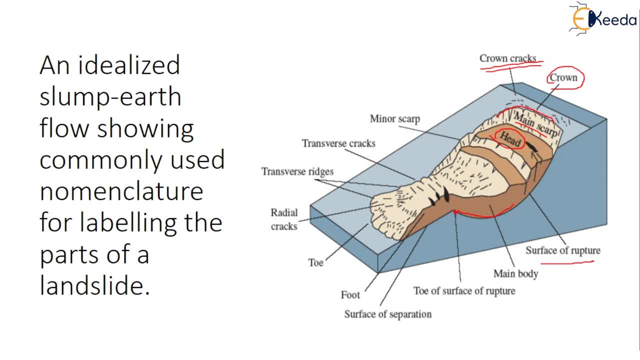 gets slided And this one is called toe of the surface of rupture. So this is the top of the structure. This is mainly called the separation or the surface of separation, And the lower part here is known as foot And the most lower part is known as the toe. Other cracks which are 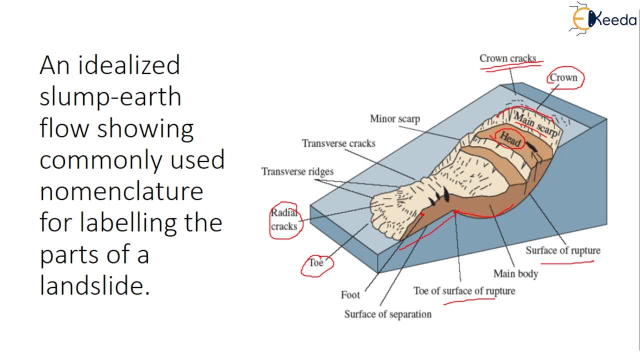 associated with the toe are called radial cracks And these are some of the transverse ridges which are associated with the toe and the foot part And these are some traverse cracks. There are also some minus cap, which is shown here, And these are some of the transverse ridges which are associated. 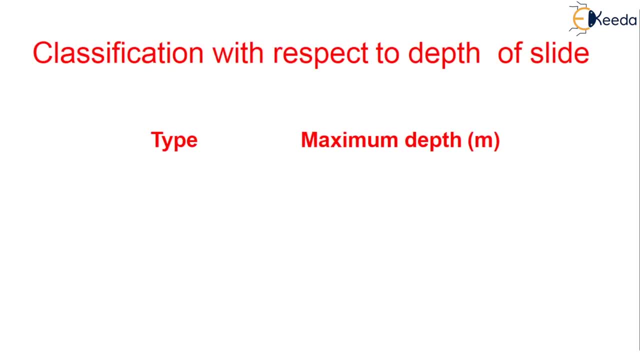 here. See after the disposition of the land Here. coming to the classification with respect to the depth of slide, Let us see what is the classification. There are actually four main types. The first one is surface slide, shallow slide, deep slide and very deep slide. Let us see. 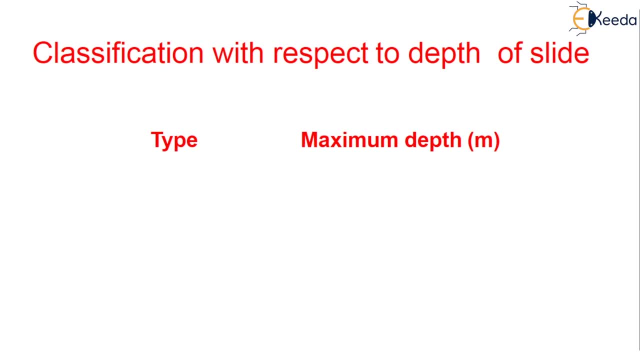 how they are differentiated with the help of the maximum depth. This maximum depth is measured in meters. The slide is set to be a maximum depth of about 3 meters, And the maximum depth of the slide is set to be a surface slide if the maximum depth is less than 1.5 meter. What is the second one? 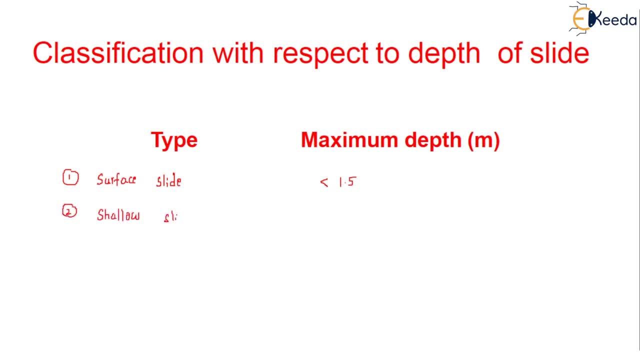 Shallow slide. Here, the maximum depth is between 1.5 to 5 meters. What is the third one? Deep slide. Here, the maximum depth is 5 to 20 meter. What is the fourth one? Very deep slide. 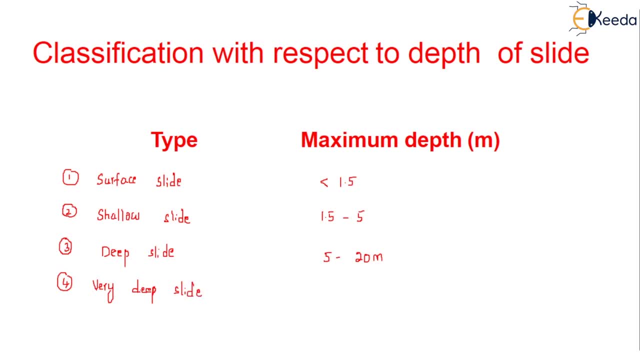 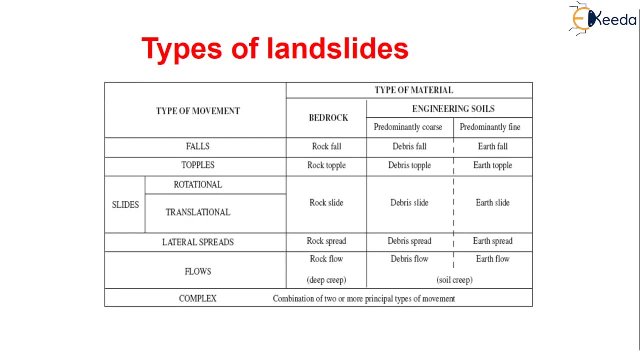 It is greater than 20 meter. See, these are all the different types of landslides, which is tabulated here. Coming to the type of movement, there are actually falls, topples and slides. Again, slides are divided into two types: rotational and translational. There are also 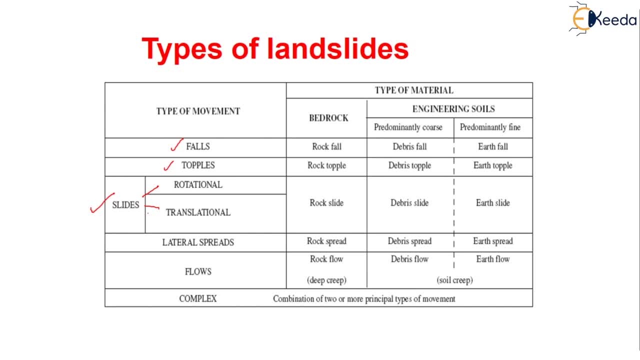 lateral splits, flows and complex. Here the type of material will be bedrock and engineering soil. This engineering soil is divided into two types, predominantly coarse and fine, Depending upon the bedrock. if it is a rock fall and debris fall and earth fall, it will be a falls. These falls are 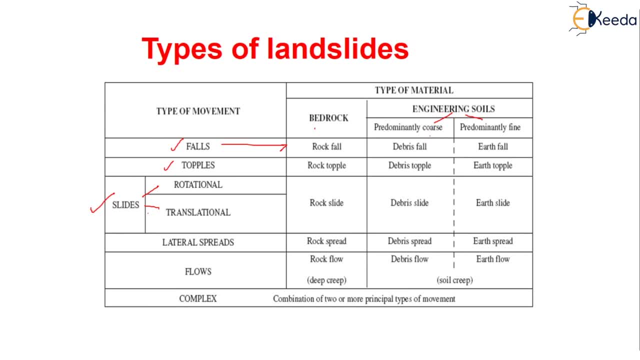 these many types: Topples, rock topple and debris and earth topple. Here slides rock debris and earth Again coming to lateral splits. rock debris and earth Flows also will be same deep creep and soil creep and complex combination of one or more above type of movements. So first one is: 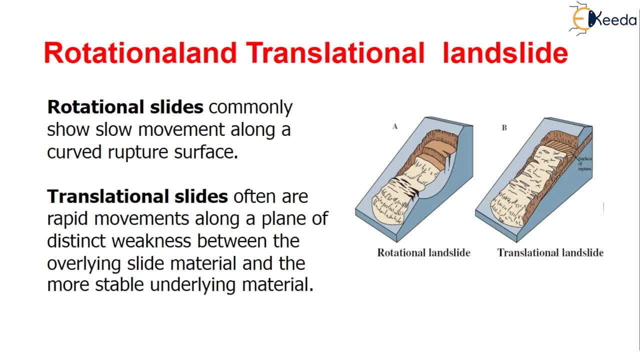 the rotation and translational landslide. What do you mean by rotational slide? It is commonly will show very slow movement, Very slow movement along the curved rupture path. Okay, it is a curved rupture path. It will show very slow Coming to the translational slide. they are actually rapid. 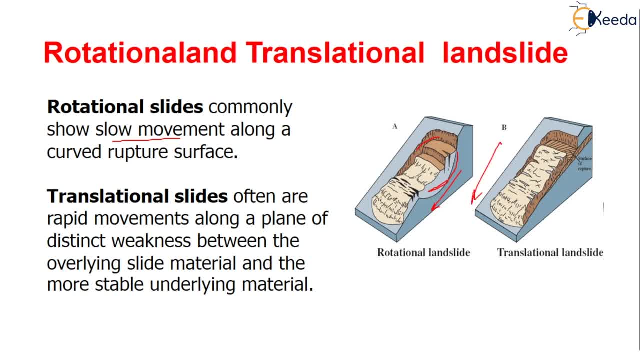 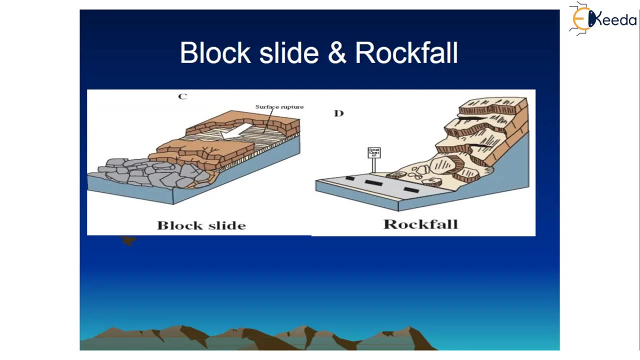 sudden, Okay, rapid. There will be sudden movement along a plane of distinct weakness between overlying slide material and more stable underlying slide metal, off from upper to the lower side- see comment- or block. slide and rock fall. this is a diagram which is showing this is a surface tuna, okay, and rockfall. it will be like this. Let me show you the 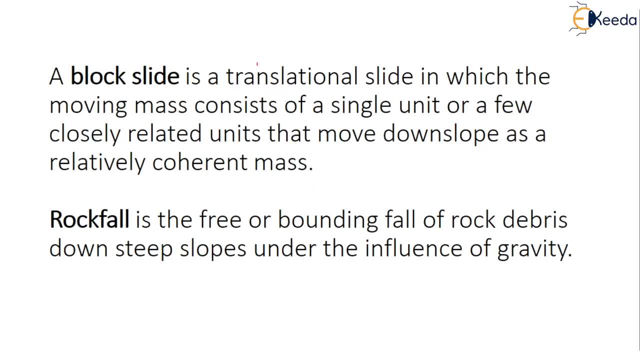 Definition generally: blocking light is nothing but the translational slide. here The mass moving will consist of single unit or sometimes a few closely related units. they generally move from downward slope as a relatively coherent mass, like the relatively 1,, 2,, 10,. 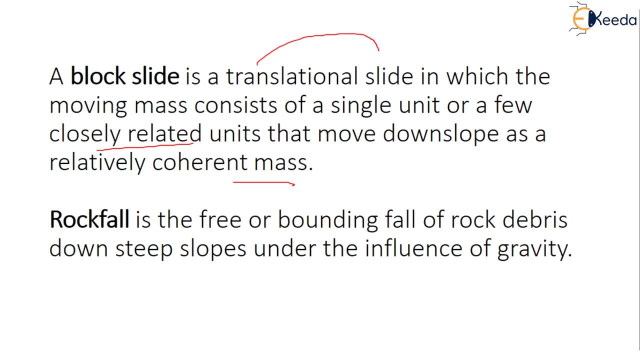 11,, 12,, 13,, 15,, 20,, 32,, 30,, 30,, 39, be moving like that, coming to the rock fall. it is nothing but a free or bounding fall of rock debris. mainly downstream slope will occur. it is mainly under the influence of the gravity. this is 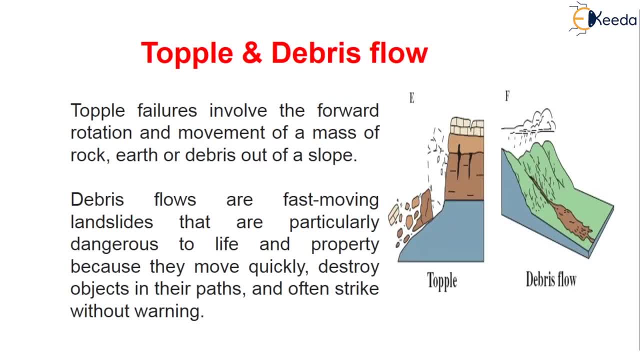 very important. okay, gravity coming to the topple and debris flow. see, this is how it looks. this topple failure will involve the forward rotation and movement of the mass of mainly the rock, earth or debris. okay, this is how suddenly it will get: forward rotation and movement coming to the debris. 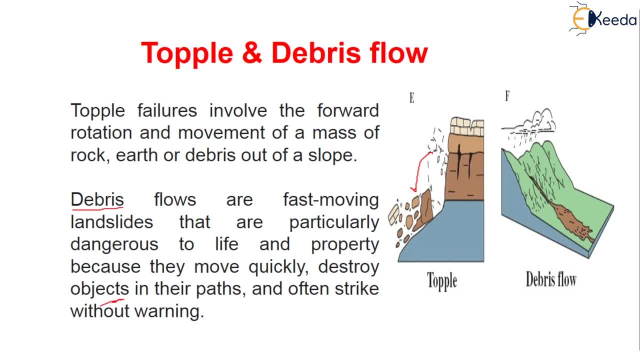 flow here what happens is in debris flow, fast moving landslides will occur- see here suddenly- which are particularly very dangerous to life and property. they destroy a lot of objects in their path and often strike without warning. there will be no warning also. this is very dangerous. 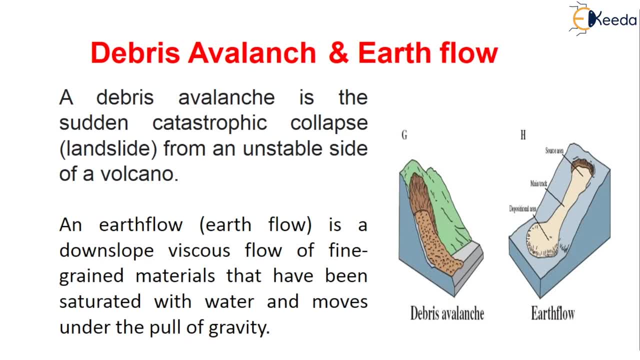 so, coming to the debris avalanche and earth flow, what do you mean by debris avalanche and earth flow? here you: a debris avalanche is nothing, but it is a sudden catastrophic collapse. it is also known as sudden falling of the landslide. it mainly comes from an unstable slide. here you can see, this is a. 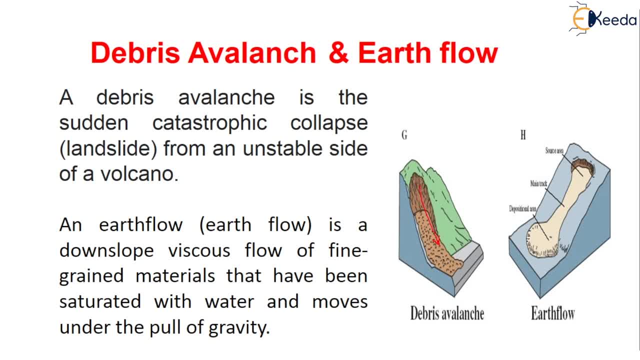 unstable slide. it will suddenly fall where it is very dangerous and there will be a loss in the property and life coming to the earth flow. what do you mean by earth flow here? it is a downslope, viscous flow of fine grained materials, so it's a very dangerous fall. 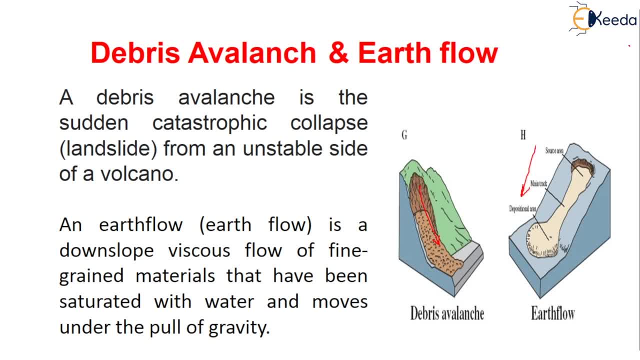 it flows like a water, like liquid. it will be a viscous flow generally, it will have saturated with water and it moves under the pull of gravity. okay, it will flow like a water, because what will flow? the water which is mixed with the grained materials will be flowing under the pull of gravity. 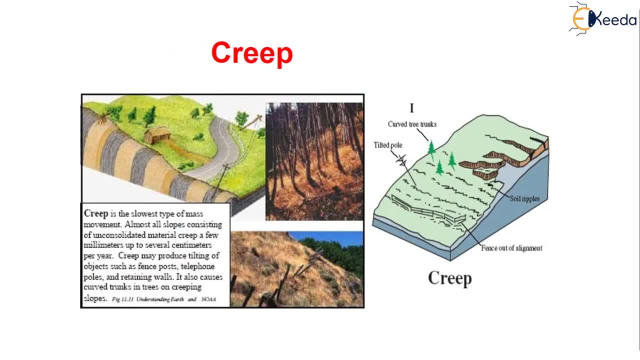 so the other one is creep. what do you mean by creep? creep is nothing but the slowest type of mass movement. it is a very slow movement of mass. almost all the slopes consisting of unconsolidated materials will creep a few mm, that is millimeters, up to several centimeters per year. it is not even visible because the movement is very. 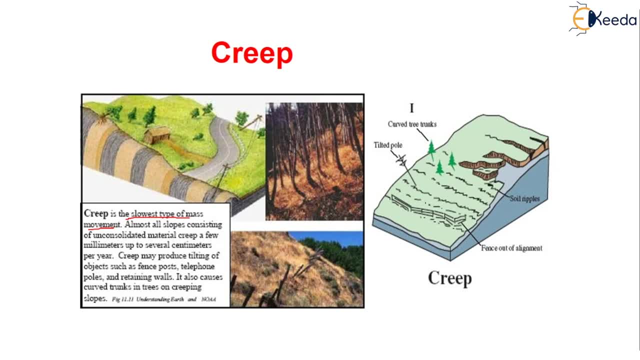 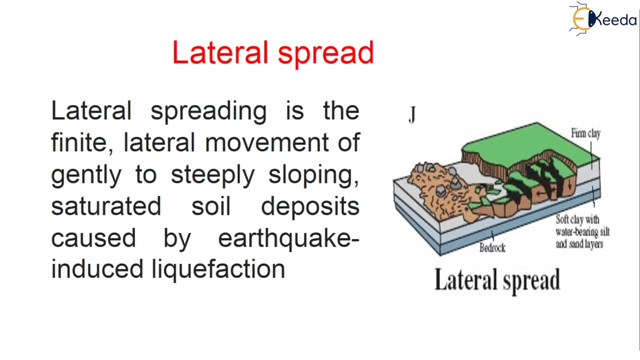 slow, so sometimes the movement will be from mm to even kilometers to centimeters. so creep may produce tilting of objects such as fence pots, telephone poles and retaining walls, because it also causes curved trunks in trees and also creep. see here: you can see, due to the creep there is a bending in the trees. 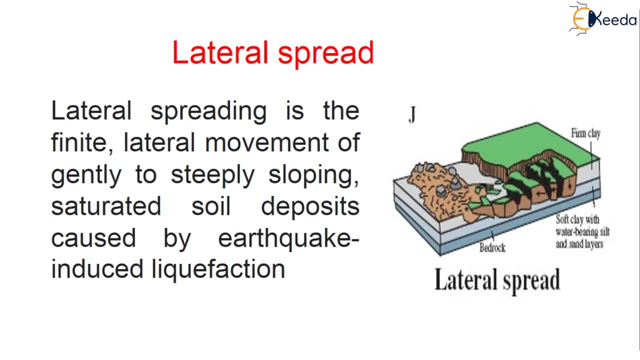 coming to the lateral spread. what do you mean by lateral spread? it is nothing but the finite lateral movement of gently to steeply sloping, gently to the steep sloping. here what happens is the saturated soil deposit will caused by the earthquake induced liquefaction like a liquefaction here. 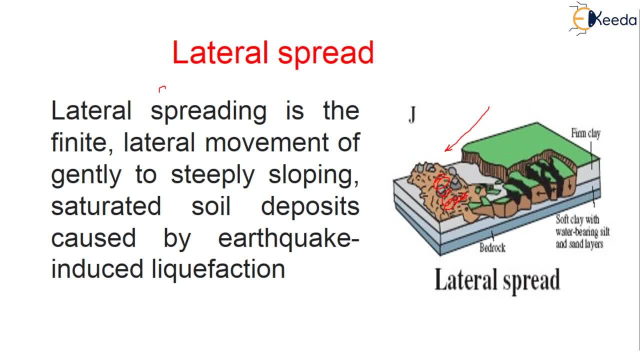 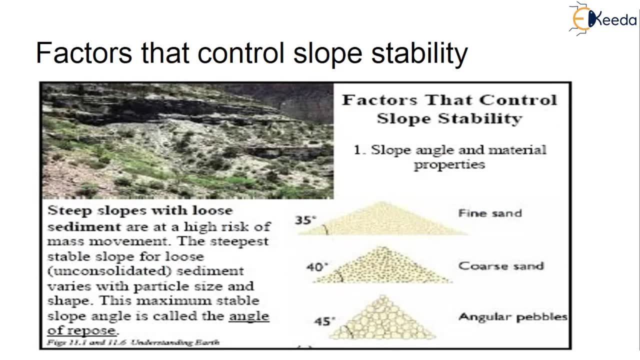 this will get flowing from gently to steeply sloping area. so there are few factors which will control the slope stability. what is the first factor? that is nothing but the slope angle and the material properties. here we have to understand that the steep slopes with loose sediment are at high risk of the mass movement that is, the mass movement will be. 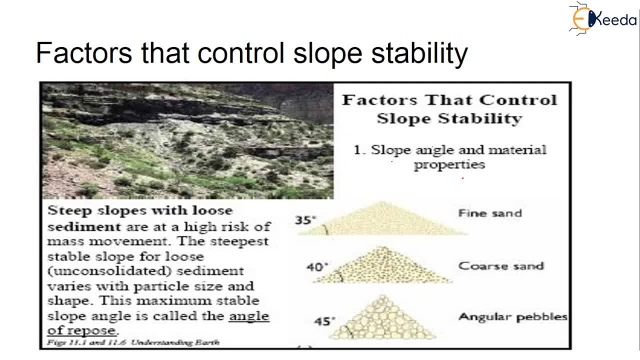 very random. that is nothing but the steepest stable slope for loose, unconsolidated material. sediment varies from practically the particle size and also the shape. so the fine sand, what is the angle? it is 35 degrees. for coarse sand it is 40 degrees and for angular pebbles it is 45 degrees. 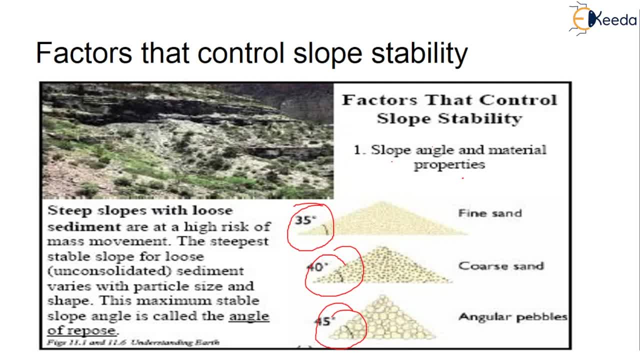 so we can very nicely tell that it is more dangerous: the fine sand. so the maximum stable slope angle is nothing but the angle of repose. so the angle of repose of fine sand is 35 degrees, coarse sand is 40 degrees and angular pebbles is 45 degrees, which is stable. 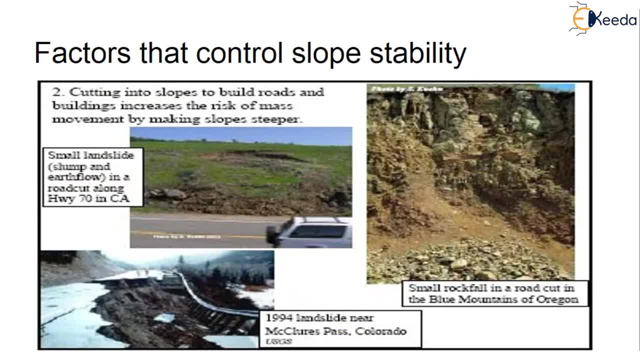 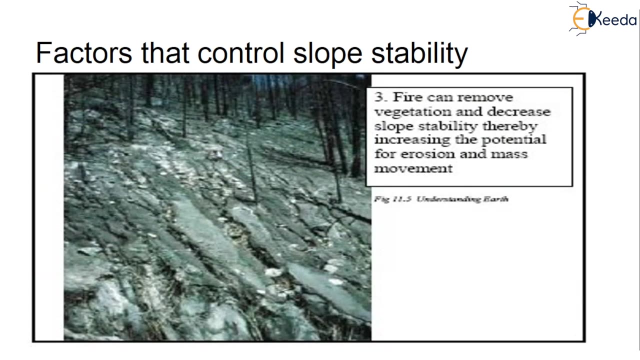 what is the second factor? that is, cutting into slope. here we have to be very careful in cutting the slopes. pick and cut wherever we want for the construction of the building, roads and buildings. so it will increase the risk of the mass movement by making slope more steeper. so one has to be taken care while cutting the slope. what is a third factor? it 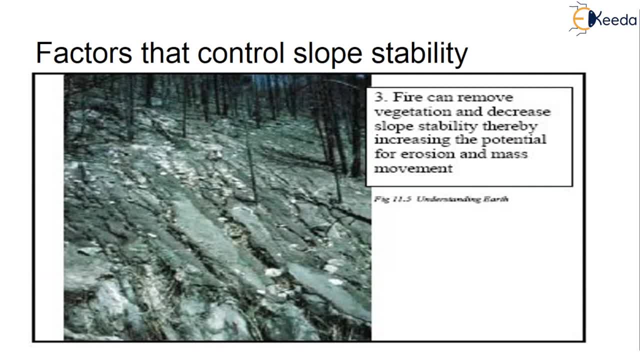 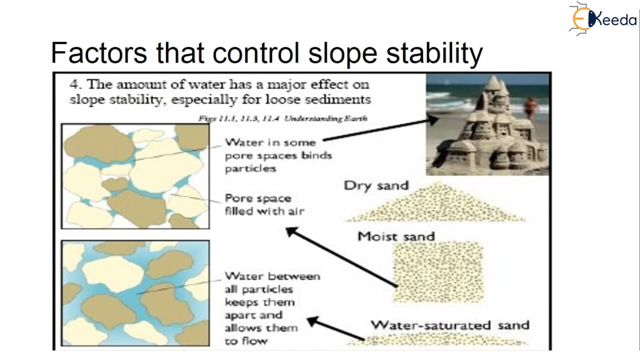 is fire, because it can remove the vegetation and also it decreases the slope stability, Therefore increasing the potential for erosion. also, mass movement will take place. So this is one of the factor which will control the slope stability. What is the fourth one? It is nothing but the amount of water. It is amount of water will play. 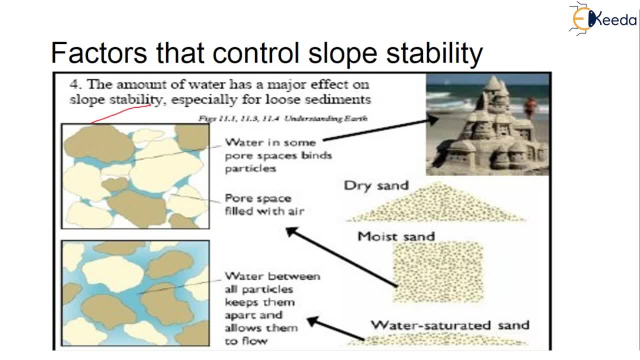 a major role which will affect the slope stability, especially for loose sediments. If you take dry sand CA, This is how it looks. Water will be in some pore spaces which will bind the particles Here. these are the pore spaces which are filled with air Coming to the water. 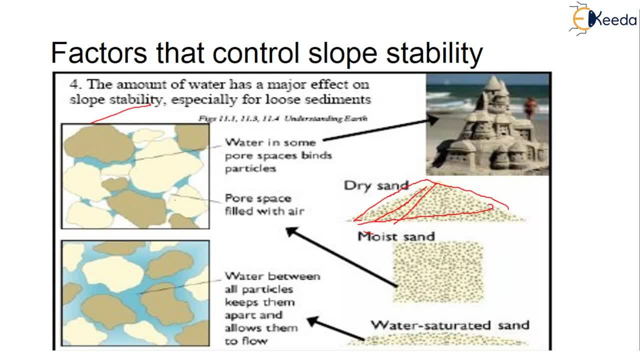 saturated sand, it will look like this. So these are the three different types which are looking. This is moist sand. This is water saturated sand: Water saturated, where water will be between all the particles, which will keep them binded okay, Which will help them. 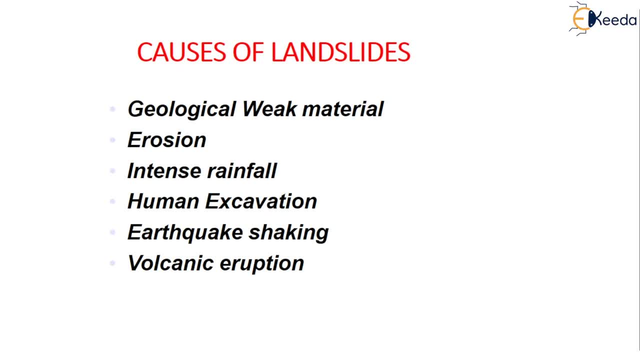 to flow. these are some of the causes of landslides. there will be like geological weak. material erosion is one of the cause. intense rainfall, human or man-made excavations, earthquake, shaking and volcano eruption. these are all. some are natural and some are man-made. these are all. 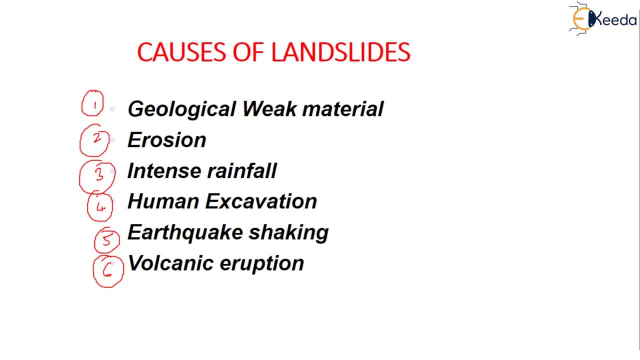 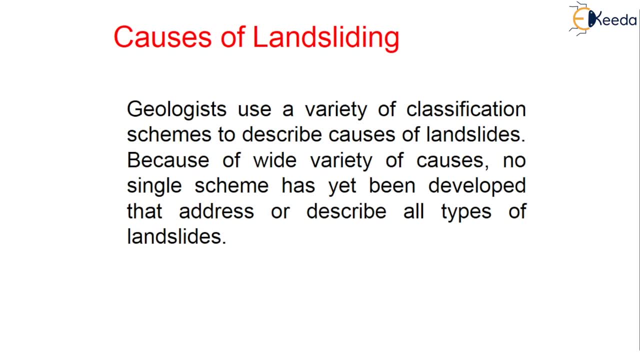 causes of landslides which are very dangerous. some can be arrested, some cannot be arrested. so the people who are giving their time and life further this subject- geologist- are using a variety of classification schemes to describe these causes of landslides. because of this wide variety of causes, there will be no single scheme, but yet they are trying to develop. 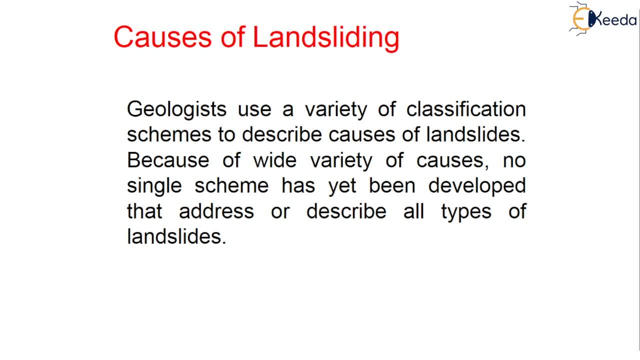 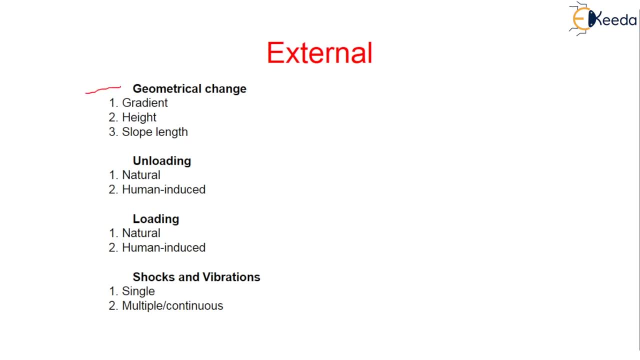 which will address all the type of landslides in one scheme. there are actually external causes where external causes we have. first one is the geometrical change. the second one is unloading. third one is loading. fourth one is shocks and vibrations. the main parts of geometrical change, a gradient, height and slope length. these are all the factors which will 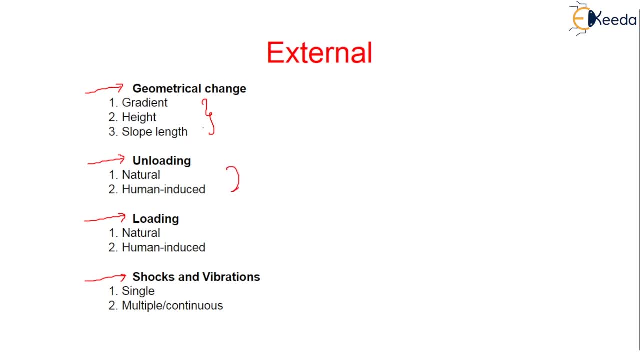 affect the geometrical change. coming to unloading. natural human induced factors are the main reasons in the loading also we have natural loading and human induced natural loading like further. naturally there will be some loading on the surface of the earth. okay, like volcano when it get a raptor like that. coming to shocks and vibrations, single and 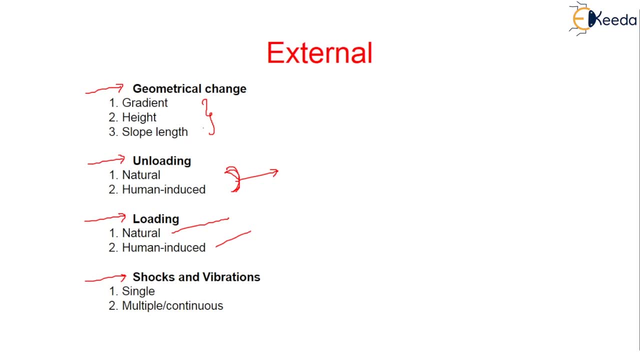 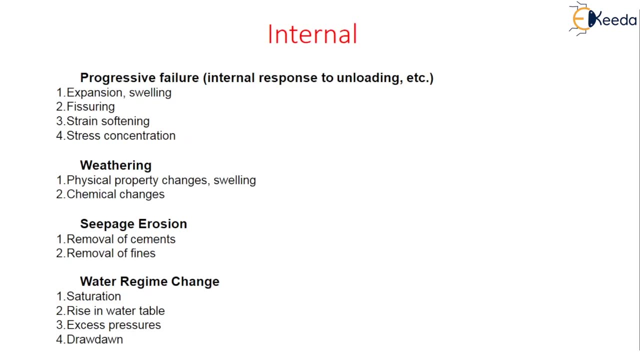 And multiple or continuous shocks may be reasons for external. During the earthquakes, during the volcanoes and during the tsunamis, we can take pills. Coming to the internal, the first one is the progressive failure. Okay, In the progressive failure we have expansion and swelling, fissuring, strain softening and stress concentrating. 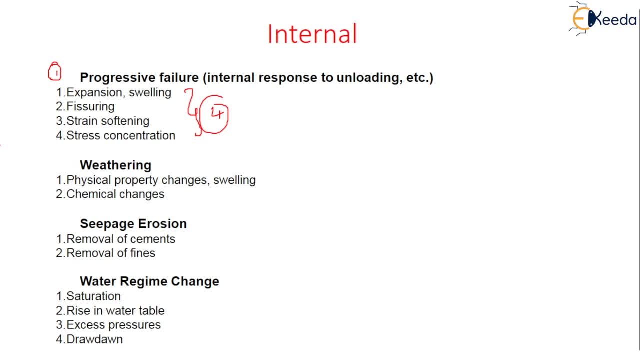 These are the four factors which fall under this failure. The second one, internal, is weather. It can be physical property changes like swelling, and chemical changes. And the third one is seepage erosion. Here removal of cements and removal of fines are the factors which will concentrate the seepage erosion. 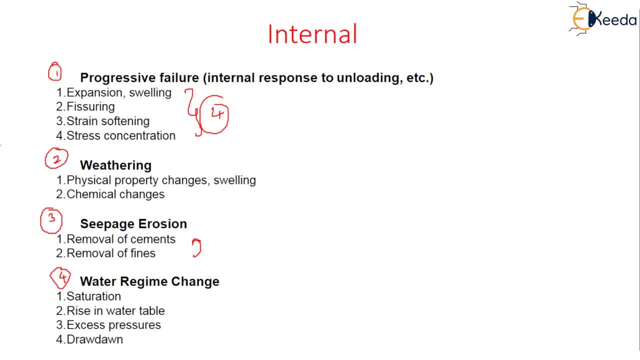 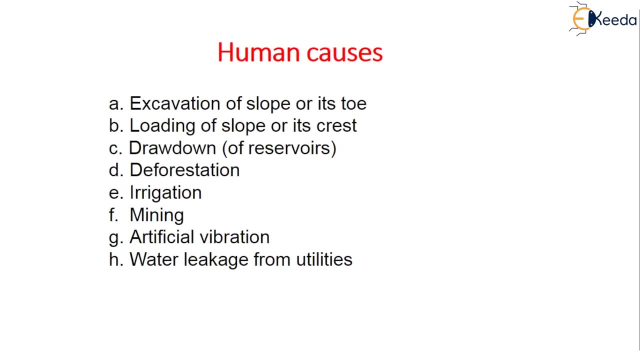 Coming to the fourth one, that is, water regime change. Here, saturation, rise in water table and excess pressure drawdown are the main reasons of water regime changes. There are also human causes, like excavation of slope, which is very dangerous, But we never know.